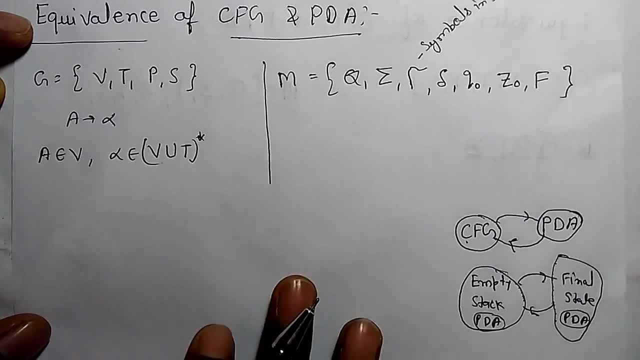 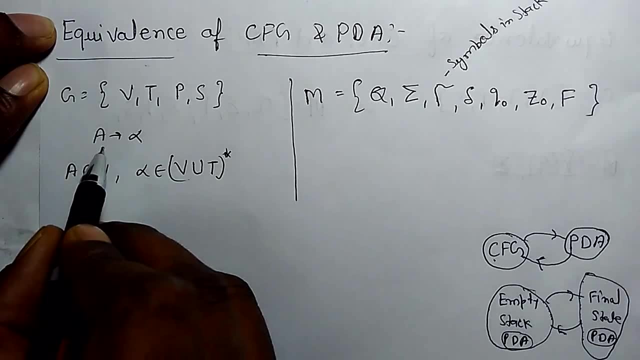 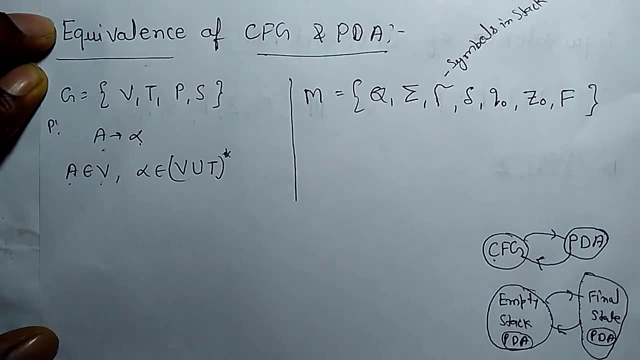 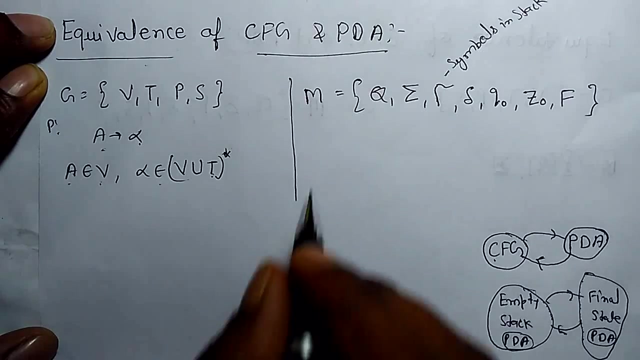 state acceptance. both are same. So this is the grammar. If it is a context-free grammar, then there should be a derivation of production rule, a drive alpha where a belongs to variable and alpha belongs to V. union T, closure. T is a terminal And there is a push-down automata. 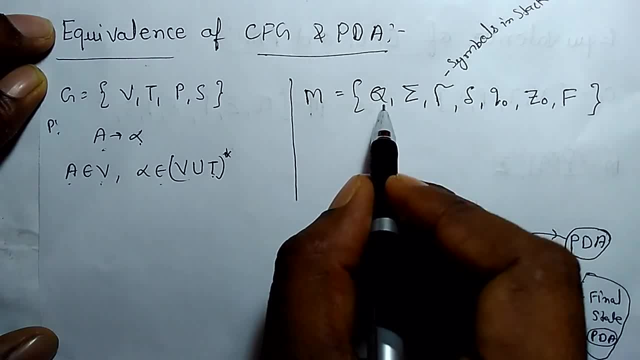 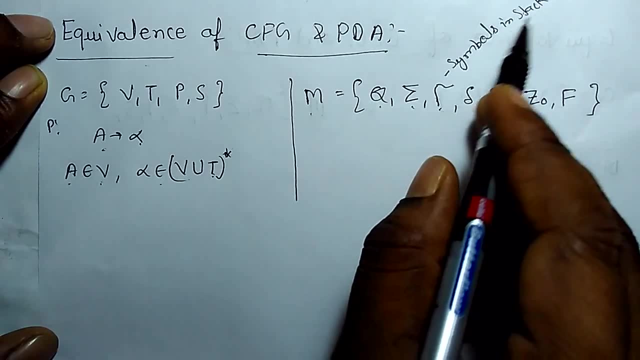 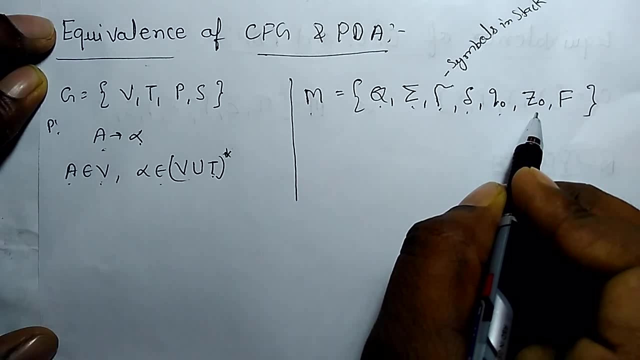 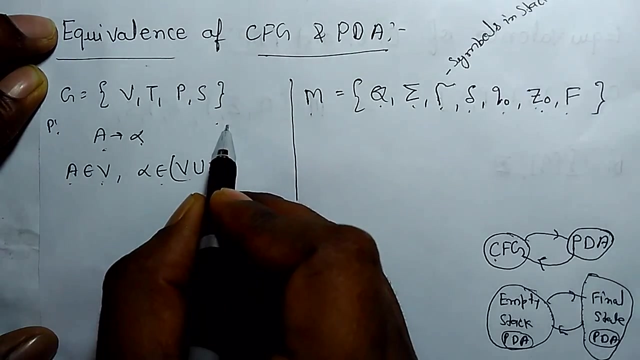 machine M, which consists of states, number of states, input symbols, tau symbols in stack transition function, start symbol, bottom of the first symbol that is inserted in this stack And final state. If we prove equivalent machine of this grammar, then equivalence of CFG to: 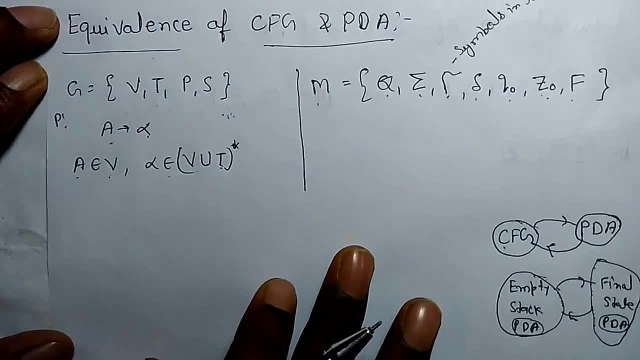 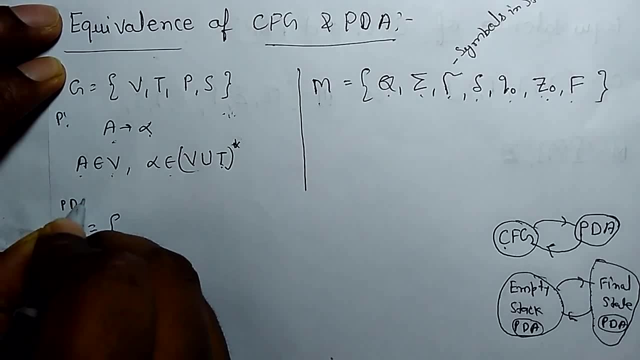 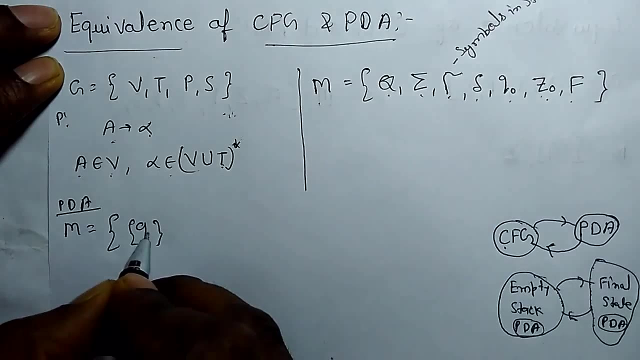 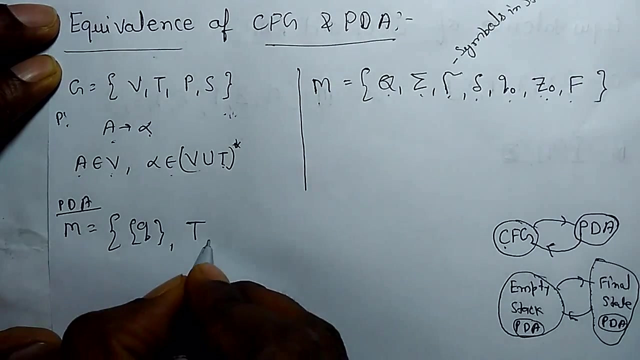 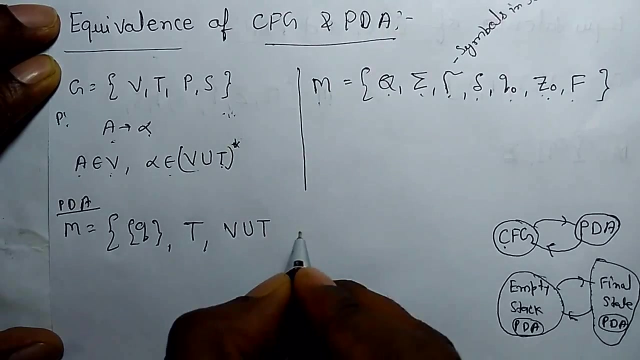 PDA is proved. So there are some assumptions. If there is a grammar, we take a machine for PDA such that number of state is only one. Q Input symbol is replaced by terminal T. Tau is replaced by V union T Transition function. 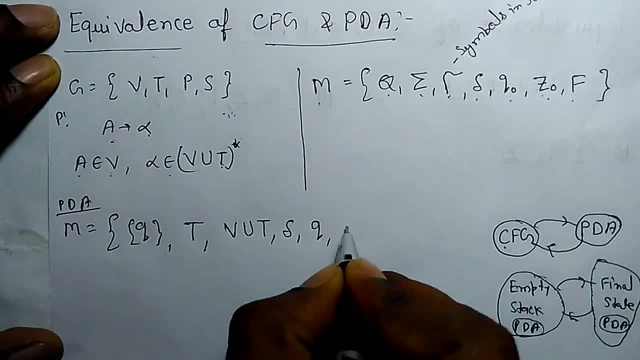 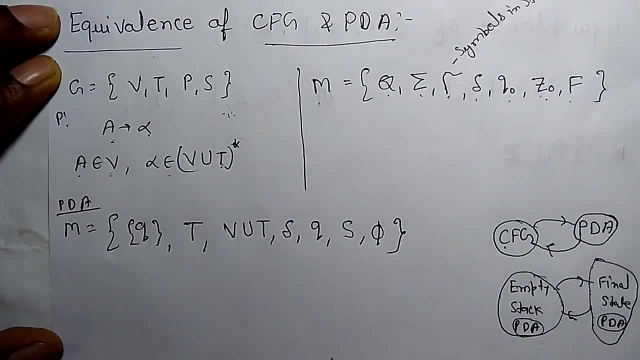 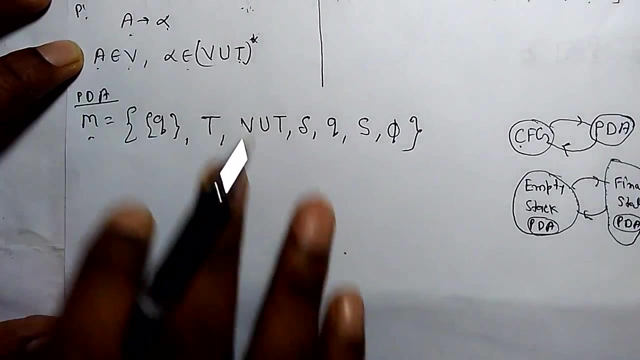 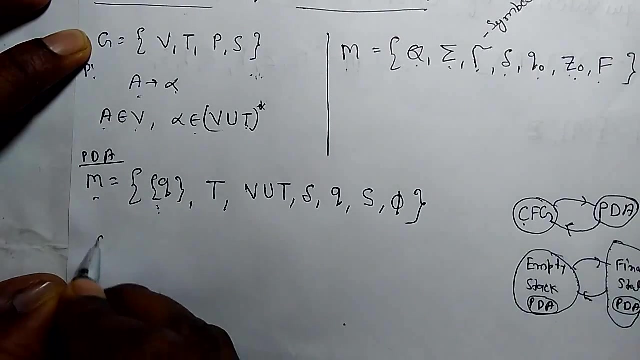 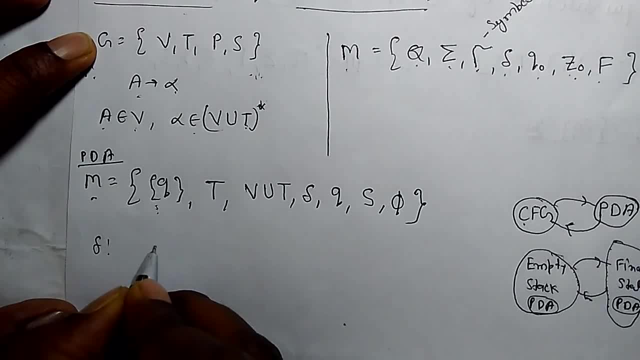 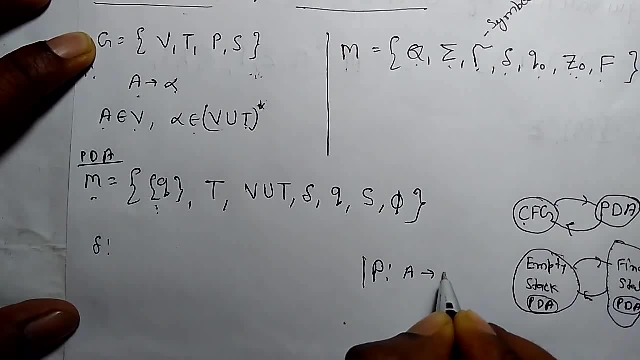 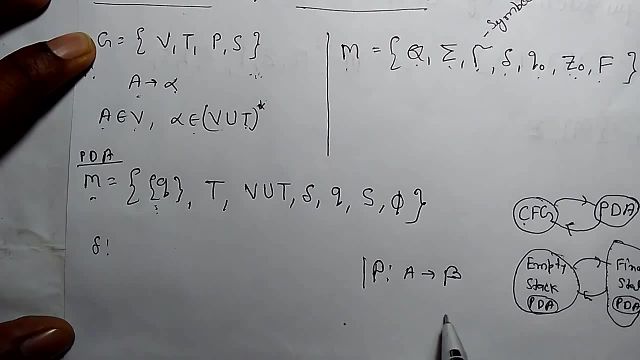 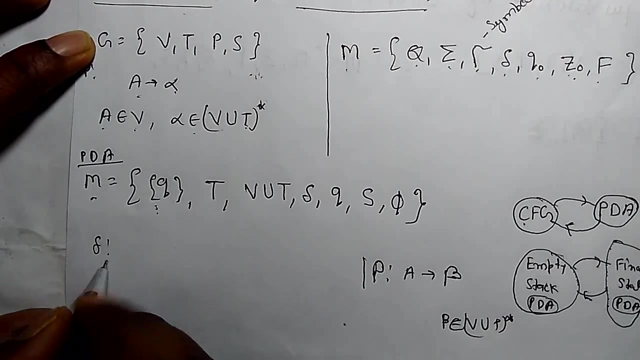 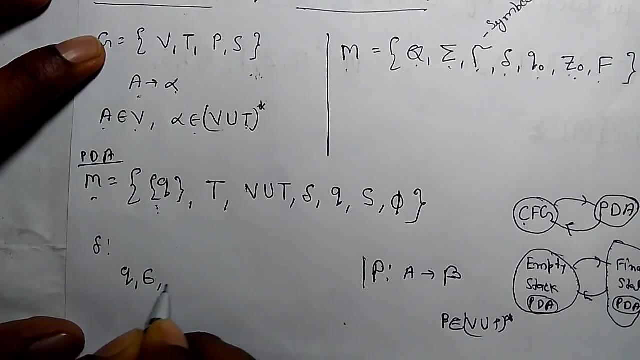 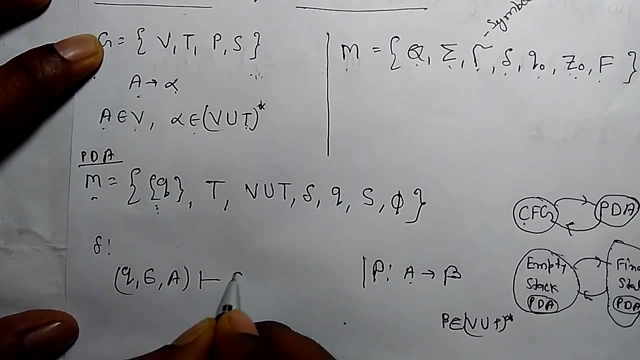 if there is a derivation in production rule, A derives beta. in production rule means beta belongs to V union, T closer. So transition function says Q. If you read epsilon, and A, which is in left side, it moves to Q and beta, which is in right side of the production rule. 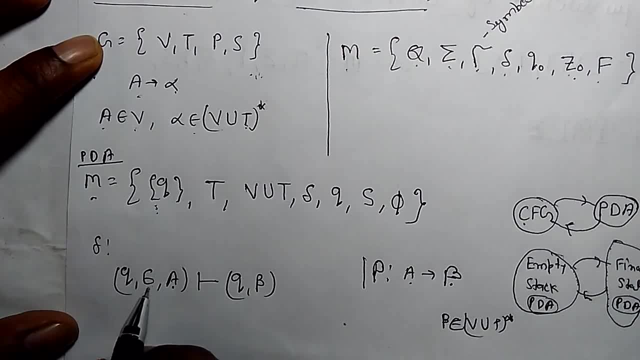 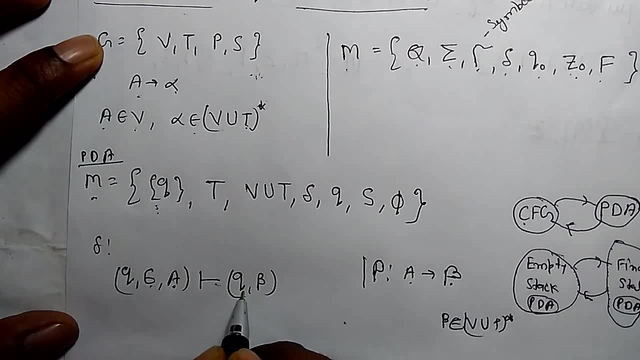 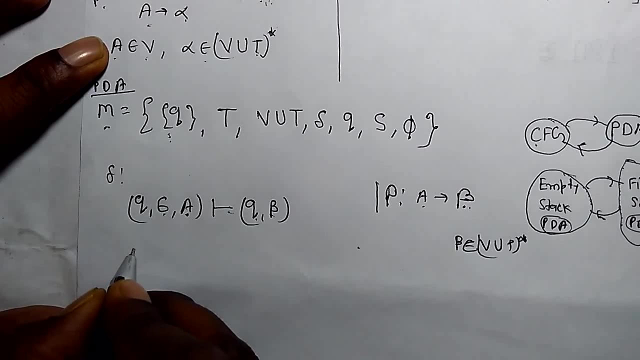 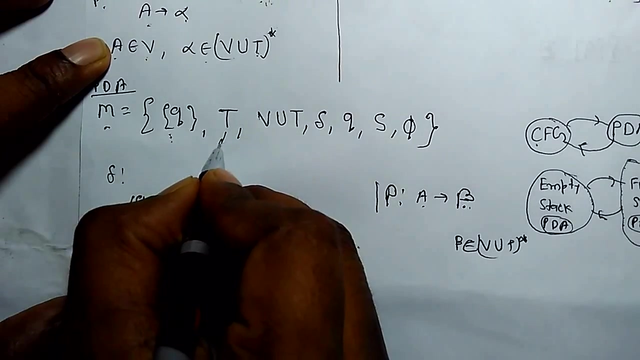 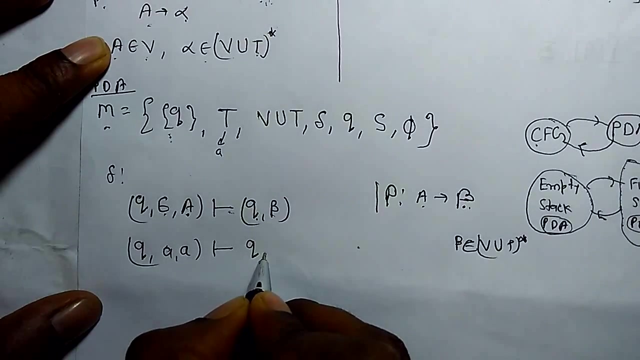 If A reads and epsilon is the input symbol, A is the top of this stack, then it will be converted into same state and right side of the production rule. Second rule, Second assumption, is if you read Q and there is a terminal terminal, for example A and A is the top of this stack, then there should be a pop operation. 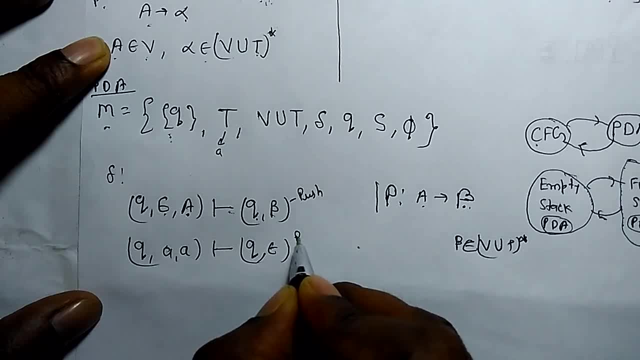 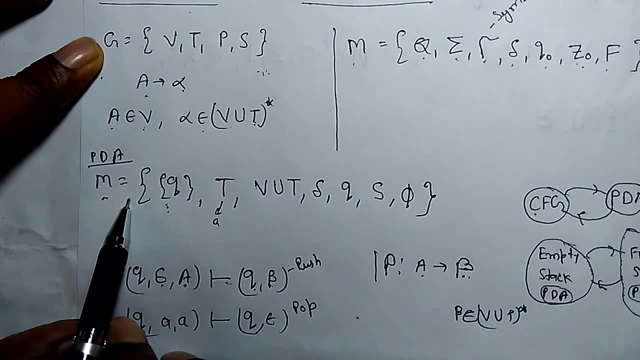 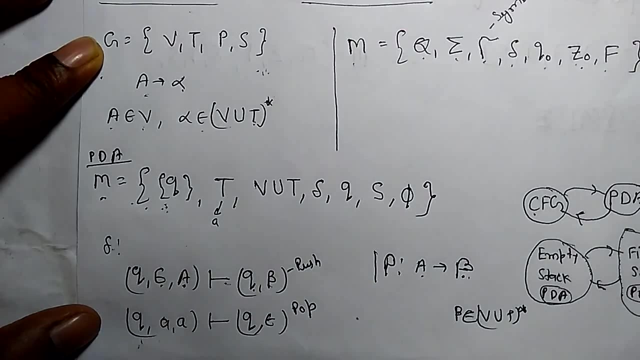 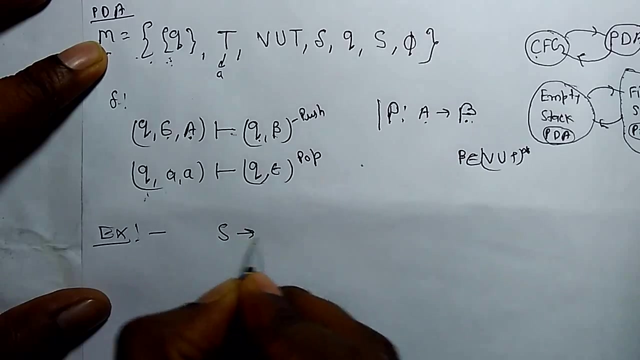 Here it is push operation, here pop. So if there is a grammar V, T, P, S in this form, We can create our equivalent push down automata where transition would be in this form. Let's take example This grammar S derived A, S, B or A B. 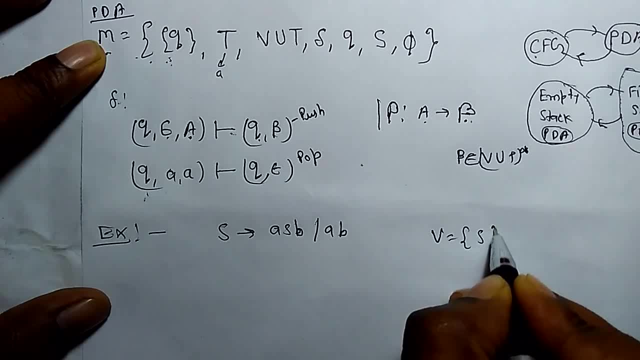 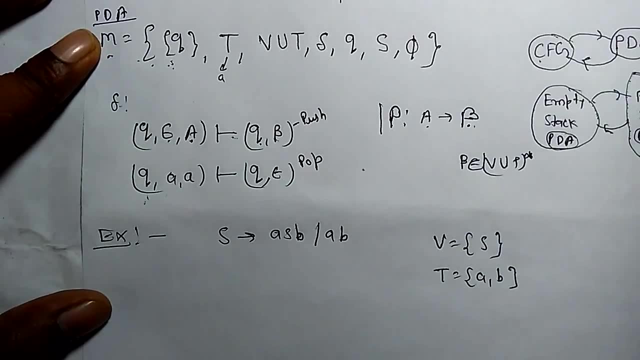 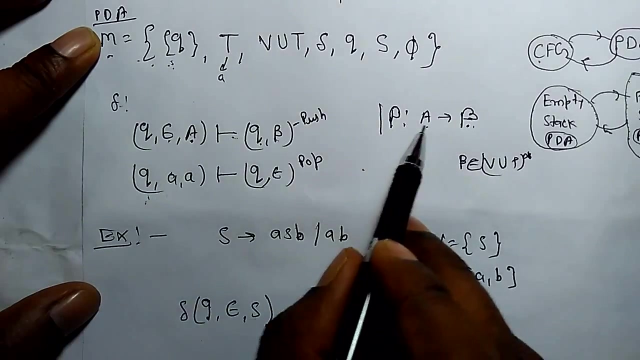 How many variables are there? Only one variable, which is S, and terminals small a and b. So for the machine we have assumed a state, Q. So transition function says: if Q read epsilon and the variable S Here total number of, you have to put all the variables at this position. 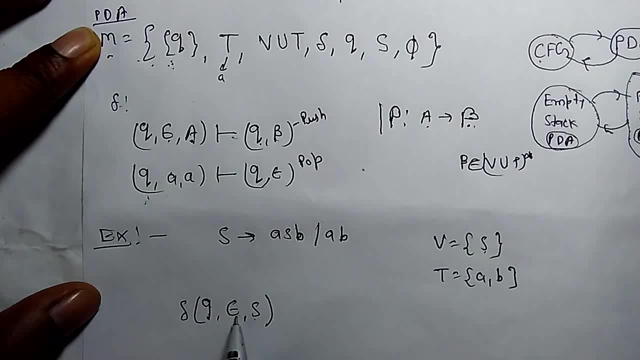 Here is only one variable, So Q input symbol epsilon. S is the variable and S is the top of the stack. This S will be replaced by right side of the production rule, So it will be Q A S B. There are two types of production of S. 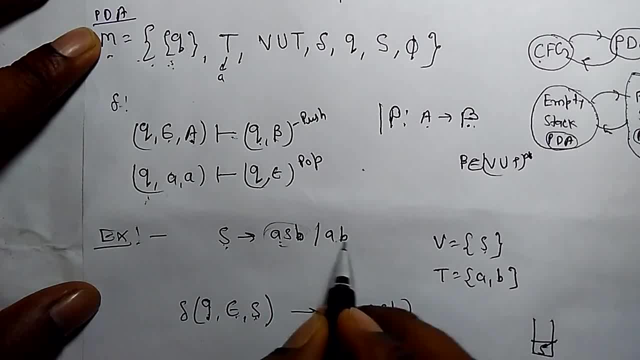 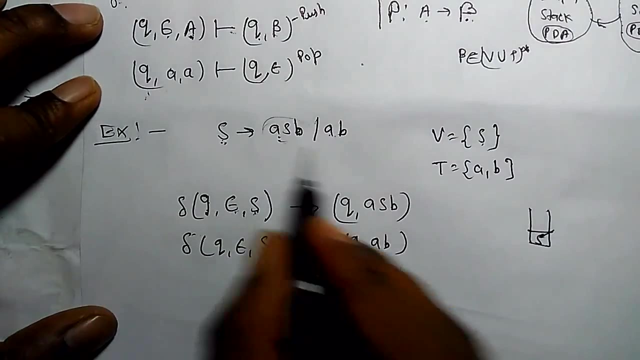 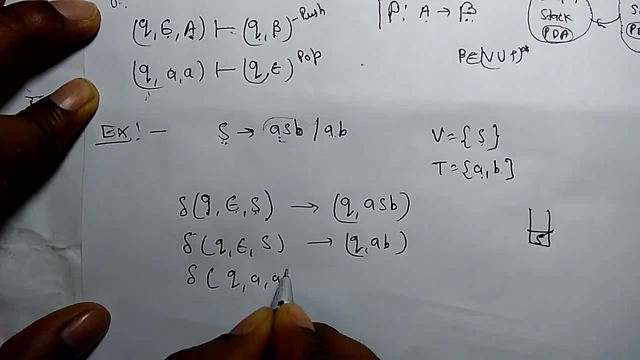 S derived A, S- B and S derived A- B. So two transition function. we write A- B. Total number of terminals are 2, A or B. For that transition would be: if A reads A as the top of the stack, Then it moves to Q, epsilon. 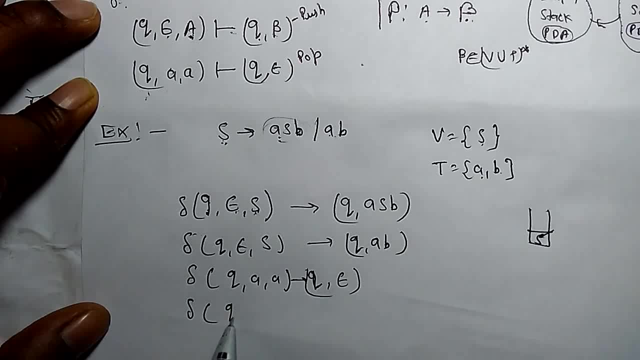 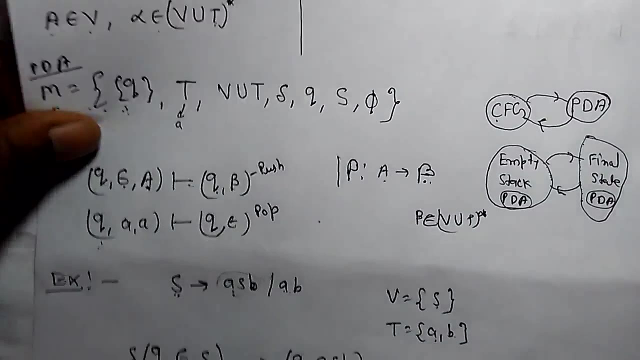 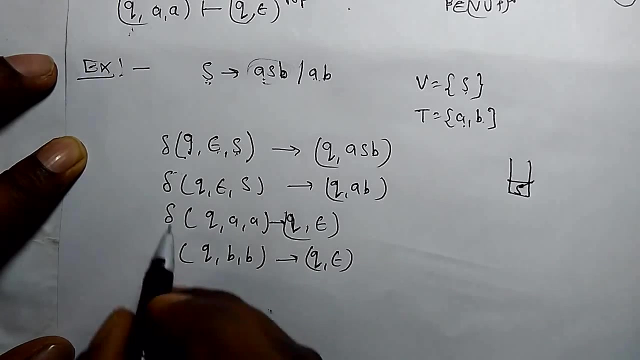 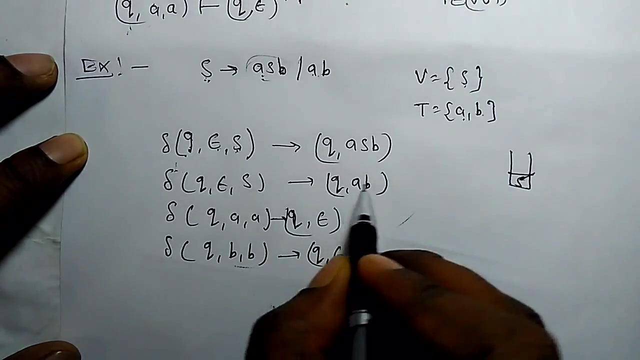 Q, epsilon, which is top. So these four transition function would be used for push down automata For PDA. we have seen total 7 terminals are there. Q is the state. Transition values are in this type. A, B are the terminals. 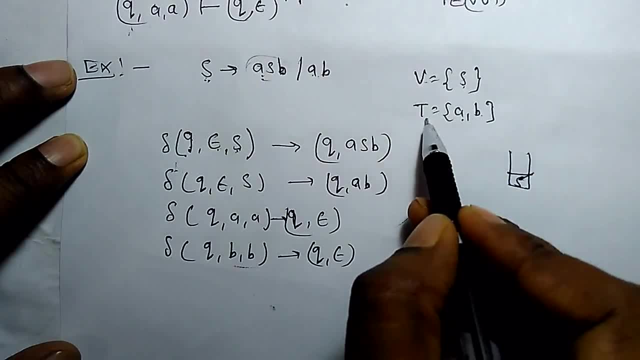 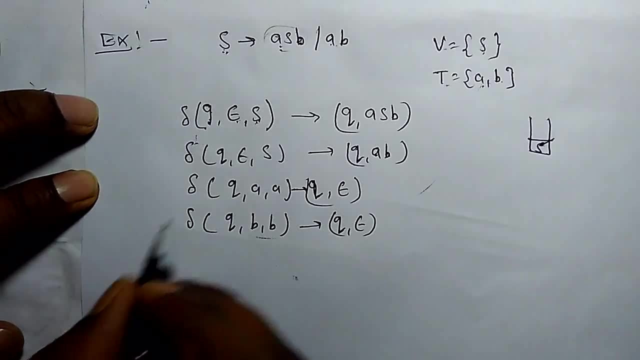 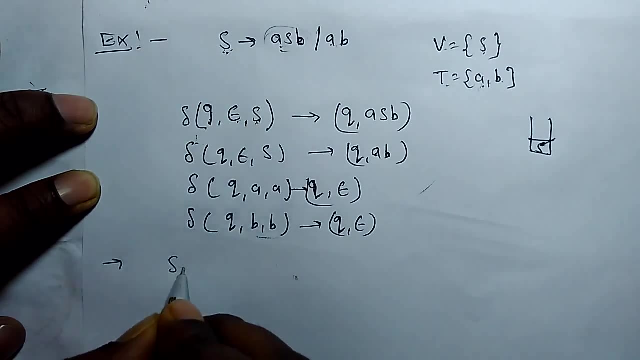 V union T. S is the variable and T is the area, So we can find the V union T. Let's take an example, One string for this grammar: If S derived A, S, B And we replace this S by terminals, The string will be generated. 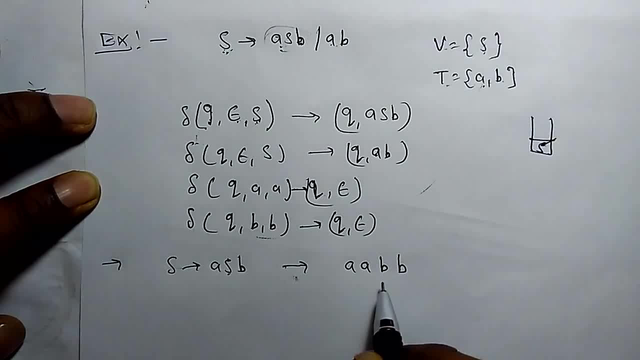 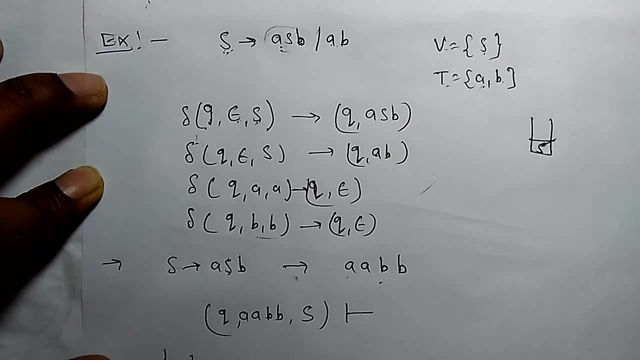 A A, B, B. Let's check where this string is accepted in this machine or not. First start with reading Q A A, B, B is the input symbol And S is the first symbol that will be inserted in the stack, So it is S. 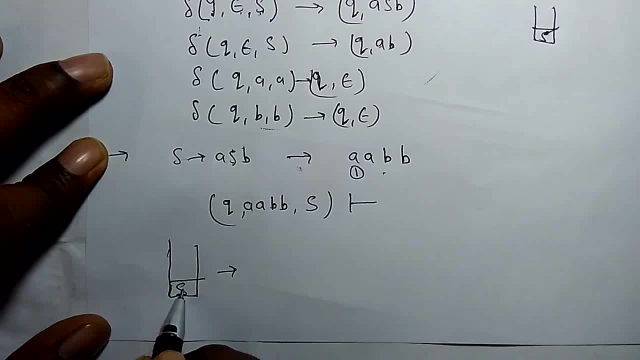 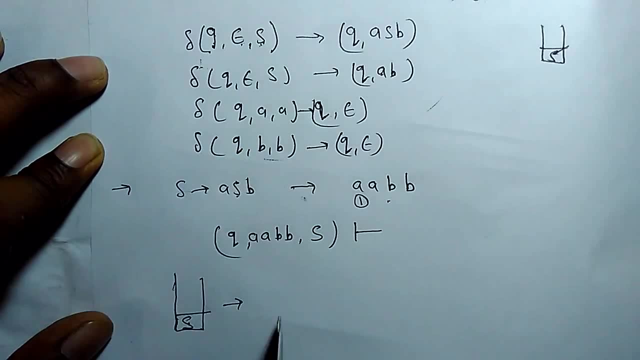 If first, if you will read. So there is not any transition, for S is the top of the stack and A is the input symbol, So we assume it is epsilon, So input symbol would be same. So this S will be replaced by A, S and B.